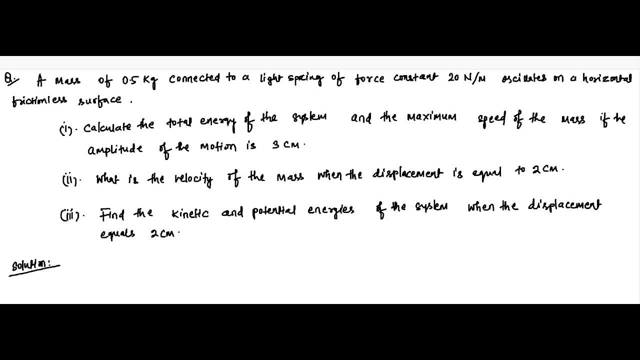 So here is another question on energy associated with simple harmonic motion. So it is given that a mass of 0.5 kg is connected to a light spring of force constant 20 Newton per meter, So it is oscillating on a horizontal, frictionless surface. We have to calculate the total energy. 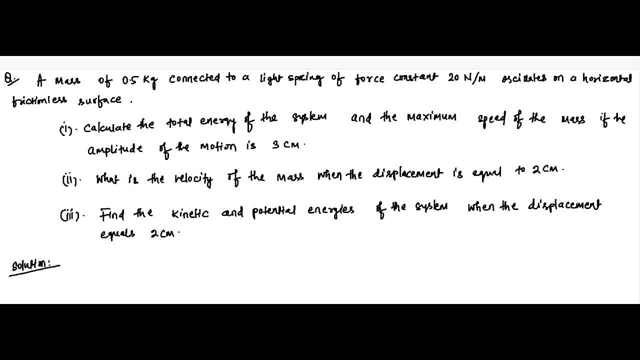 of the system and the maximum speed if the amplitude of this SHM motion is 3 centimeters. Second bit: we have to find the velocity of the mass when the displacement, the instantaneous position, is equal to 2 centimeter, And we have to find the kinetic and potential energies of 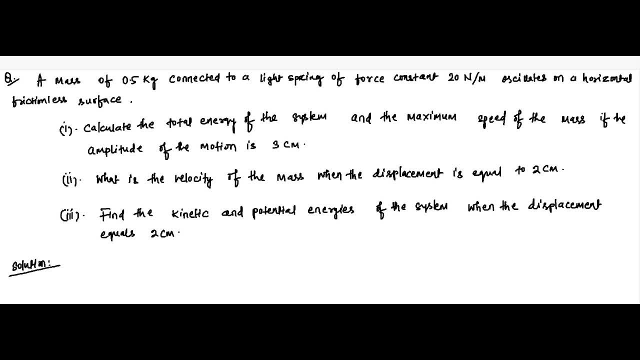 the system for the same displacement that is equal to 0.5 kg. So this is the first bit. So it is given that a mass of 0.5 kg is connected to a light spring of force constant 20 Newton per. 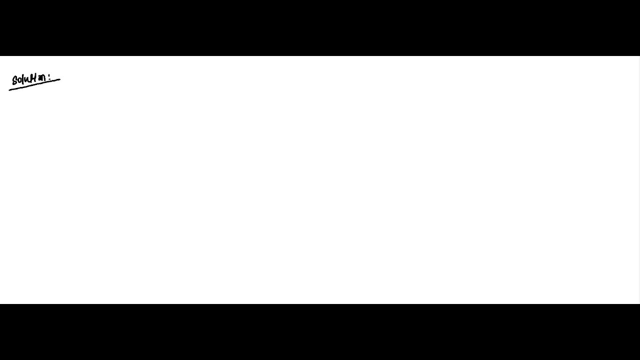 meter. Okay, So this is the whole thing. So we have a horizontal frictionless surface. On that we have a mass, let us say an object of mass m which is connected to a spring. Okay, So let us say this is the equilibrium of the object which is connected to a spring. 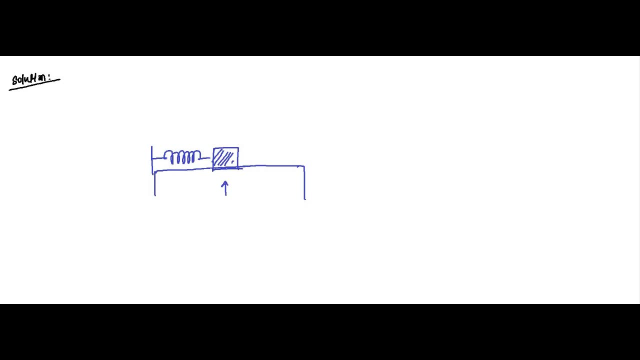 Okay. So let us say this is the equilibrium of the object which is connected to a spring position. okay, so here it is moving in a horizontal position. so let's say this is the equilibrium position and this is the maximum it can go either way. so that is equal to 3 centimeter, and here minus 3 centimeter, like that. this is the thing. mass is equal to how much? 0.5 kg spring constant k is equal to 20 newton per meter. okay now. first it has been asked to calculate the total energy. now we know that the total energy is equal to the potential energy. 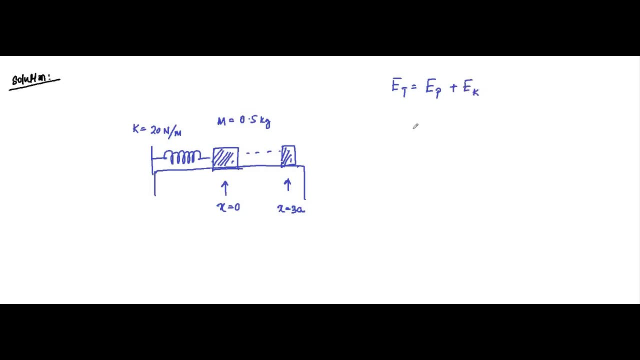 okay, plus kinetic energy at any position. so that is equal to 1 half k x square, which is the potential energy, and 1 half k a square minus x square. so 1 half k x square minus 1 half k x square. they get cancelled out, so it becomes 1 half k a square. here the amplitude of oscillation a is equal to 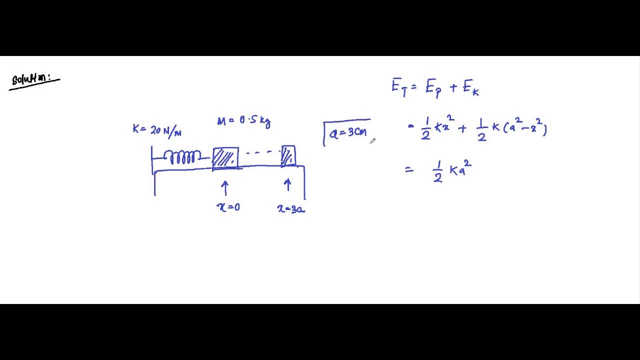 3 centimeters. okay, a is equal to 3 centimeters, so the total energy is this much. we simply have to substitute a with 3 centimeter, that is 1 half into k, 20, into 3, into 10, to the power minus 2, converting it into meter. so it becomes: 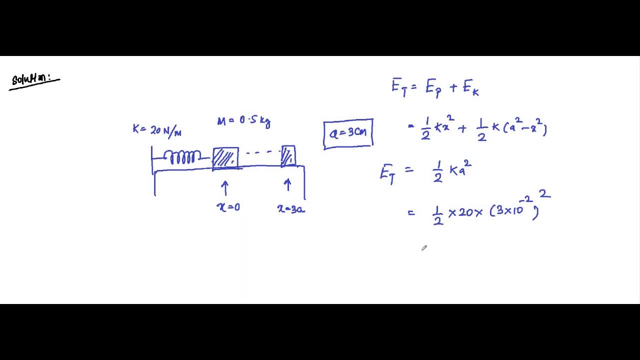 9 times, 9 times to 10, to the power minus 3 joules. this is the total energy, okay, which is constant, always constant throughout the shm motion, which we have discussed many times in the previous questions too. next, in the same bit, it is asked to find the maximum speed. okay, there are two ways we can. 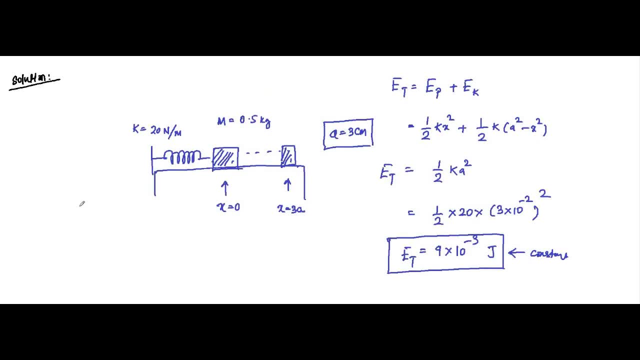 do this. i will show you both. first is the straightforward way. we know that for shm the maximum velocity or speed that is equal to omega into a is the amplitude. omega is the angular frequency. here omega is not given, so we have to calculate it. so omega is equal to: 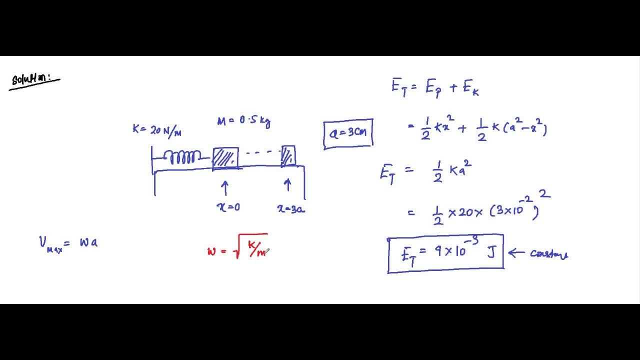 root over of k by m spring constant by mass, root over equal to 20 by 0.5. so which is basically equal to root over of 40 radians per second. so just coming around, if we calculate the decimal value, it is coming around 6.324 radians per second. now 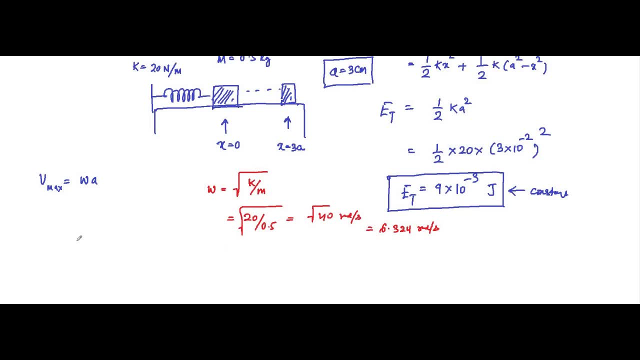 the maximum speed or velocity will be equal to 6.324 into a amplitude which is 3 centimeter, converting into meter 3, into 10 power minus 2, that is equal to it is coming 0.19 meter per second. so this is the first way. another way we can do this is c. 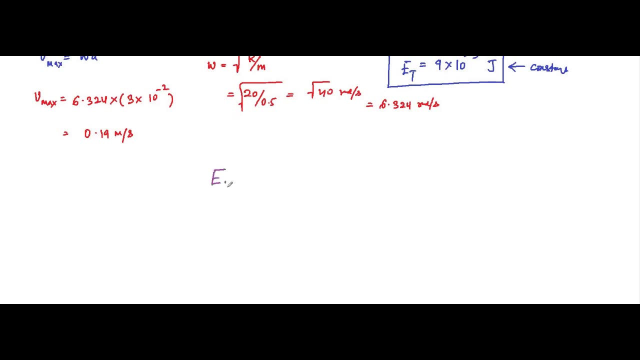 the kinetic energy. it will have maximum value when velocity will be maximum. okay, when velocity will be maximum maximum, okay. now, when kinetic energy will be maximum, the maximum value at that point, potential energy will be zero, zero joule. but the sum of the kinetic energy and potential energy, it is always constant, that is. 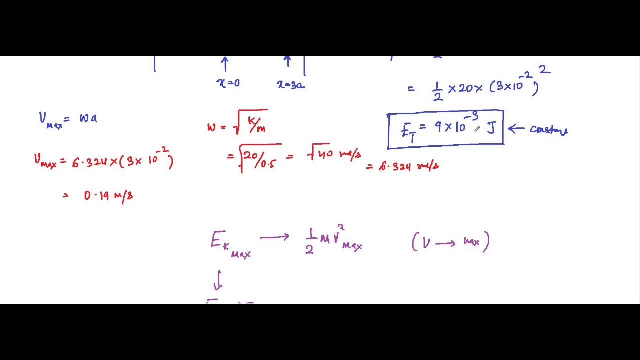 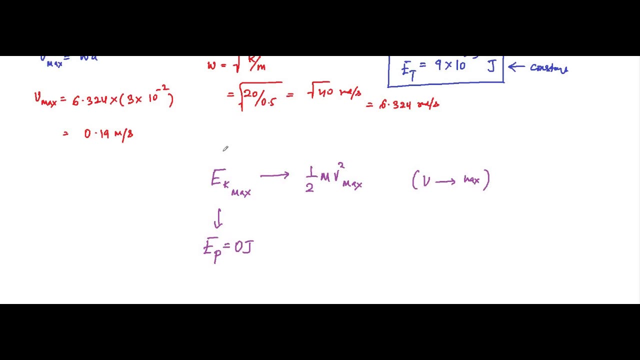 equal to 9 into 10 to the power minus 3 joule, which means that when the kinetic energy is maximum, its value will be equal to 9 into 10, to the power minus 3 joules, which means one half mass of the body, which is: 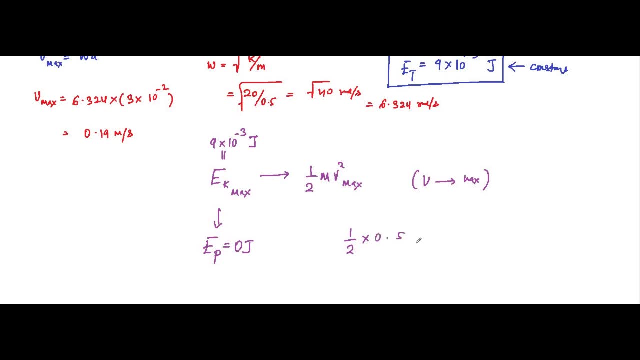 0.5 kg into V square max is equal to 9 into 10 to the power minus 3. that implies V square max is equal to 9 into 10, to the power minus 3 into 2. by 0.5 or V max is equal to root over of. 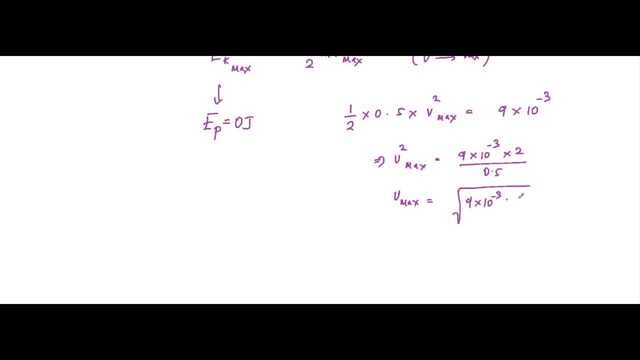 the above thing, that is, 9 into 10 to the power minus 3 into 2 by 0.5. ok, Yes, So this becomes how much that is equal to also 0.19 meter per second. same thing, ok, This is also same. 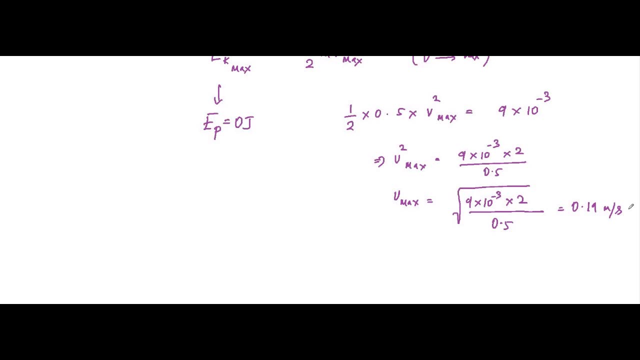 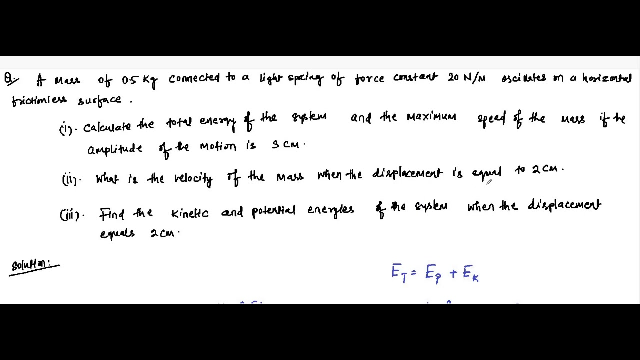 So here. So both ways We are getting the same value of maximum velocity. So either way you can proceed. Next it says it has been asked to find the velocity of the mass when the displacement is equal to 2 centimeters. 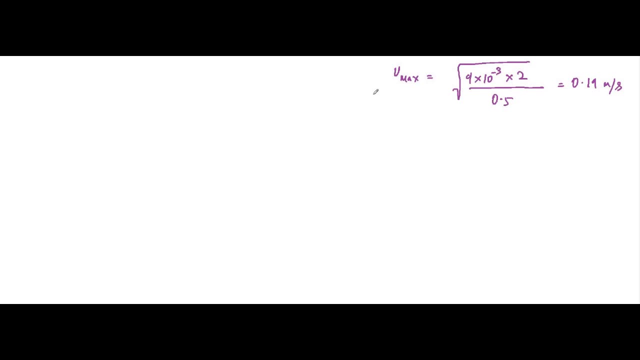 So here we know the basic formula. at a particular position, velocity is given by omega into root over of a square minus x. square a is the amplitude, X is the instantaneous position, omega is the angular frequency. Angular frequency value of, calculated it is 6.324 radians per second, into a, the amplitude. 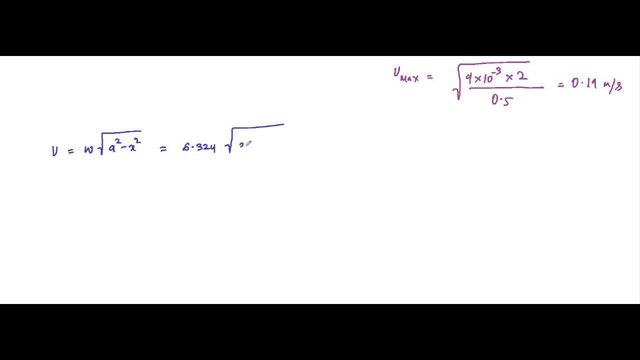 which is 3 centimeter, 3 into minus 2 whole square, minus 2 into 10 to the power, minus 2 whole square. So this is the amplitude, So this is the amplitude. So this is the amplitude, Whole square. ok. 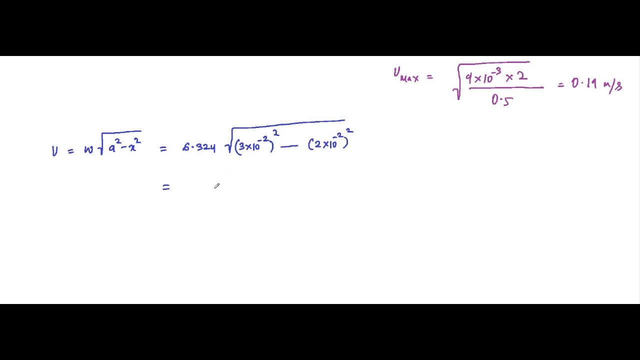 This much, So it is coming around 0.14 meters per second. ok, This Then. it has been asked to find the kinetic and potential energies of the system when the displacement equals 2 centimeters. So this is the second bit. 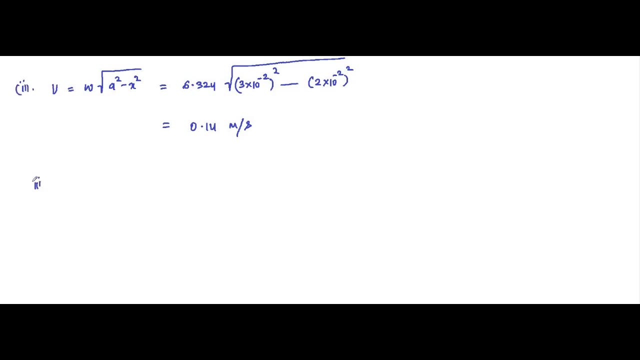 And then the third bit, the kinetic and potential energies of the system when the displacement is 2 centimeter. So potential energy, we all know 1 half kx square equal to 1 half. which is equal to how much? 20 Newton per meter? that is the spring constant, I think yes, 20 Newton per meter. and x square is 2 into 10 to the power minus 2 whole square. 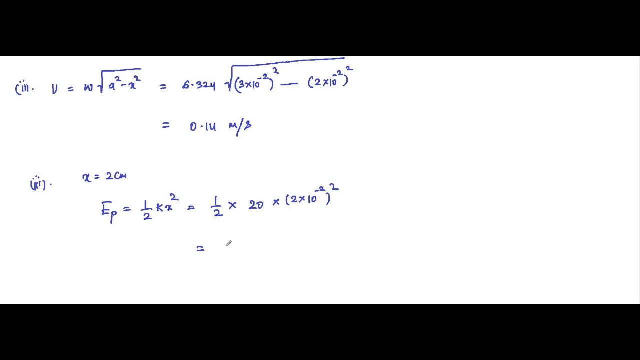 So it is coming around 4 into 10 to the power minus 3 joules kinetic energy, that is equal to 1 half k a square minus x square, equal to 1 half into 20 a square, which is equal to 3 into 10 to the power minus 3 joules.